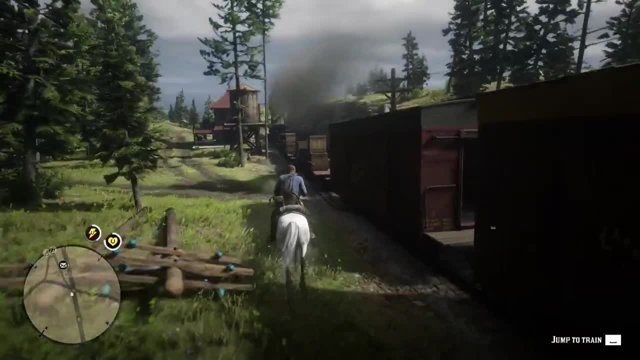 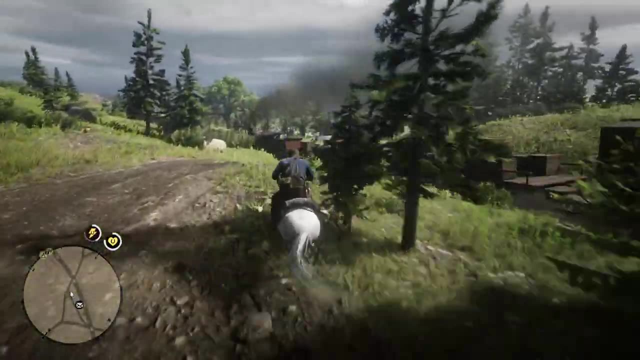 two completely different time periods. The iron horse epic is referring to the small-scale regional development of the railroad system which would allow people to settle further away and extend a hinterland of the CBD, And the steel railway system was referring to the transcontinental 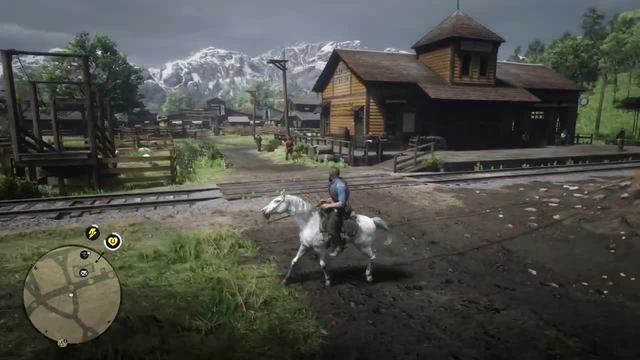 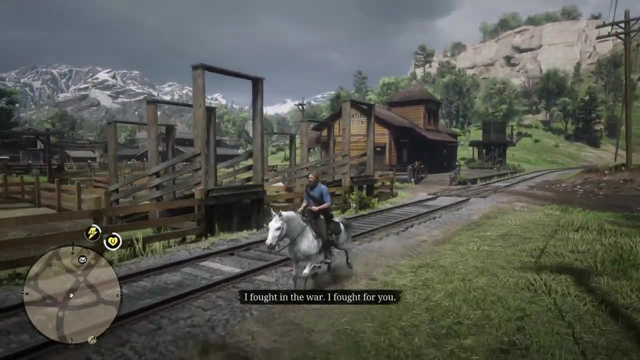 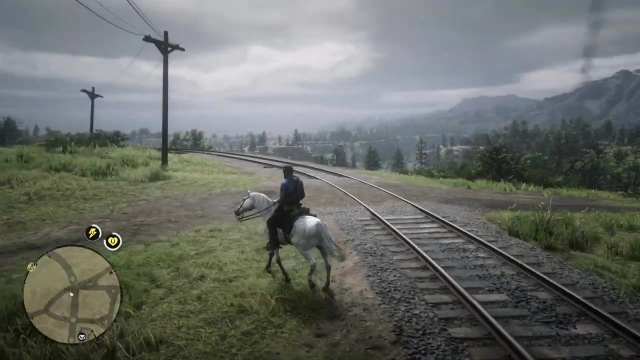 railroad system. So look at a town like this, for example. It developed closer to CBD. You see the small-scale development of towns along the railroad tracks as a byproduct of the iron horse system which, technically speaking, extended the hinterland further than the wagons, But it was shorter than the transcontinental. 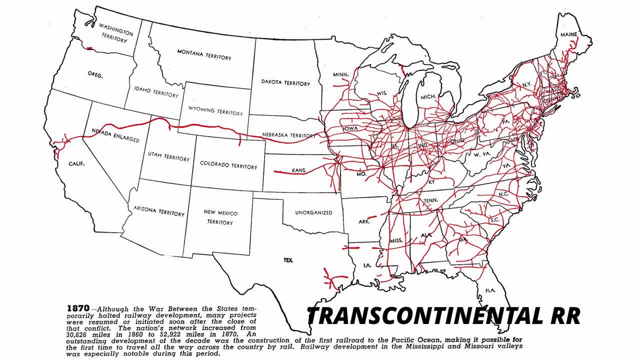 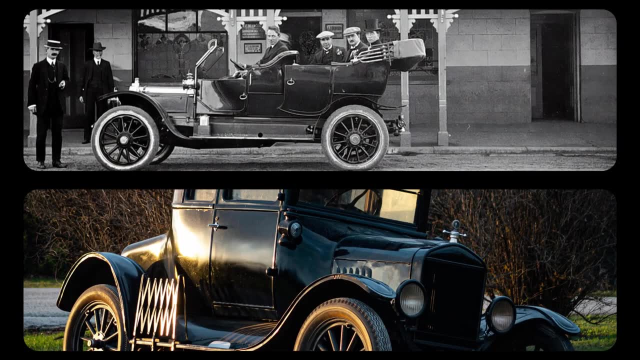 railroad system which was completed in 1869. And this system allowed urban areas to develop and thrive in the Midwest, particularly cities like Kansas and Omaha. Then you have the automobile epic, which actually looked more like this with the Model T, And this freed the people from the 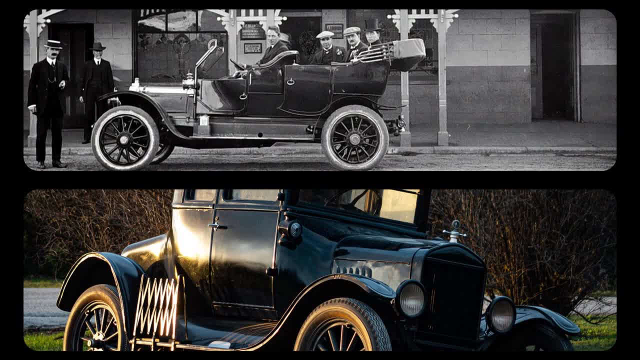 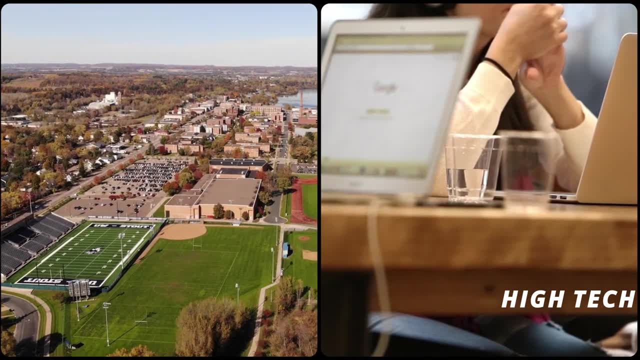 railway system and eventually allowed for suburbanization to occur. And last but not least, you have the fifth epic, which is the iron horse system, which actually looked more like this with the high-tech epic, And this originally wasn't a part of Borchert's model, but was added later on. 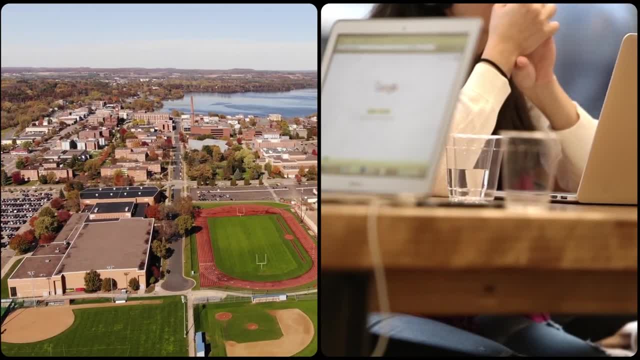 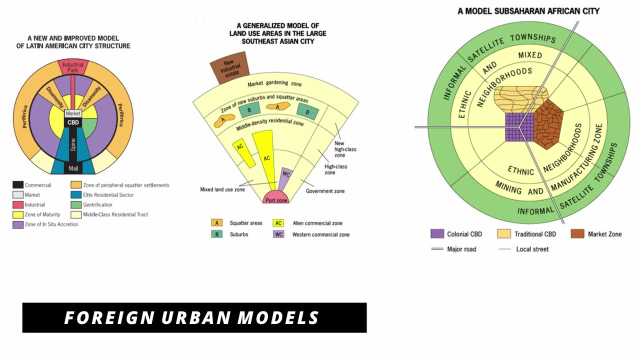 And this stage is referring to the development of urban areas around colleges and universities and high-tech industries like Silicon Valley. And, as promised, let's look at the foreign urban models. And with these three models, there are a few common denominators. First off, 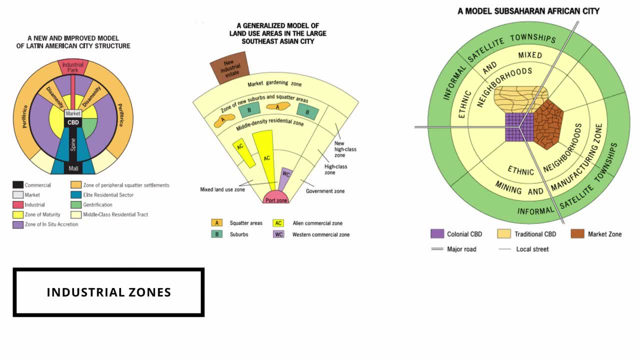 you're going to see that all three of the models have an industrial or manufacturing zone which is going to be closer to the poor regions, Once again reiterating the idea that pollution and access to work contributes to the location. You also have various translations of a traditional CBD for each one, For example: 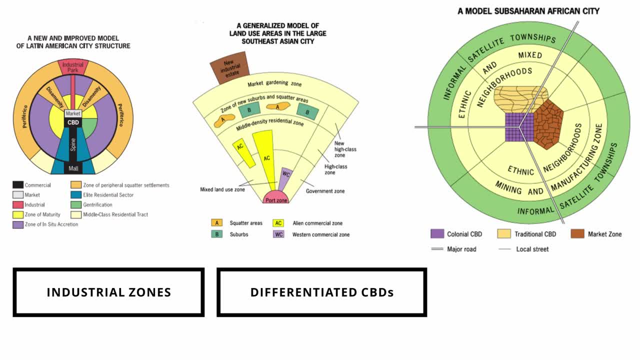 the Latin American city model has the market, the CBD in the spine, the Southeast Asian with their port zone and the three different CBDs for the Sub-Saharan African city. Lastly, you will see the similarities between the Latin American and the Sub-Saharan in that you have roads and freeways implemented directly within the model itself. For the Latin, 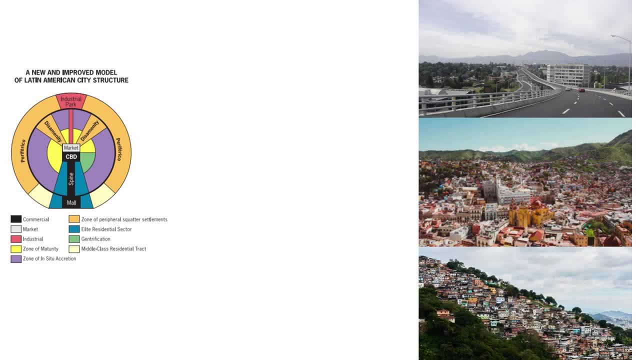 American city model. we want to recognize that it starts on the outside with the squatter settlements, AKA the favelas, which is a map on so many video games, And as you move further in you're going to see the transition zones, which includes the zone of maturity and in-situ. 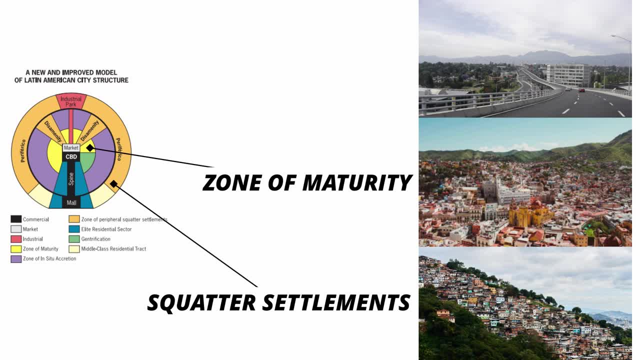 accretion And towards the center, you have your upper class in the spine and it implements gentrification, which is something we will discuss later, And this entire model is connected with the periferico, which is the freeway system. The Southeast Asian city model is unique in that it's 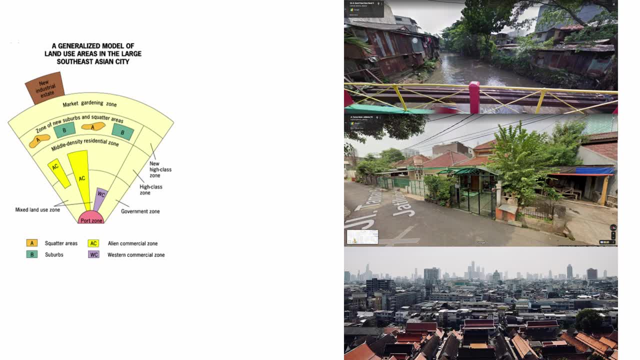 mixed classes, which is something you don't see often in urban models, as you'll note that the squatter areas in the suburbs are mixed together, And you can even see this in Google maps. If you go to Jakarta, Indonesia, the first two pictures are actually just right down the street from one 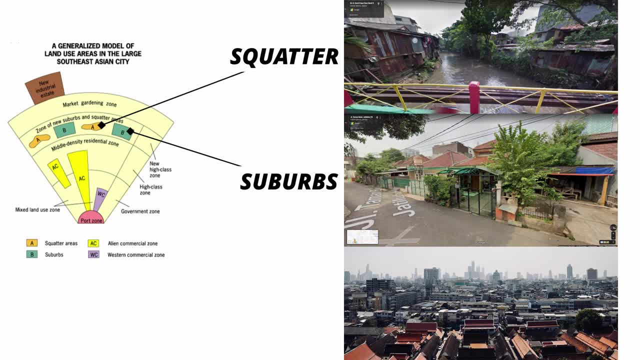 another, And in many regions of the city you'll see this mixture of the lower and middle class. Then it's important to recognize the foreign and colonial influence, with the alien and commercial zones. And, lastly, this model is unique in that you have your port zones as your CBD, which is 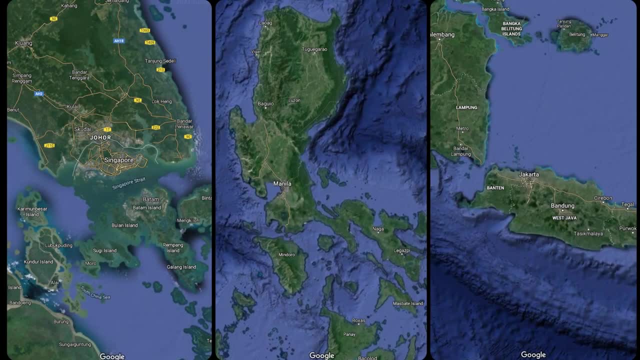 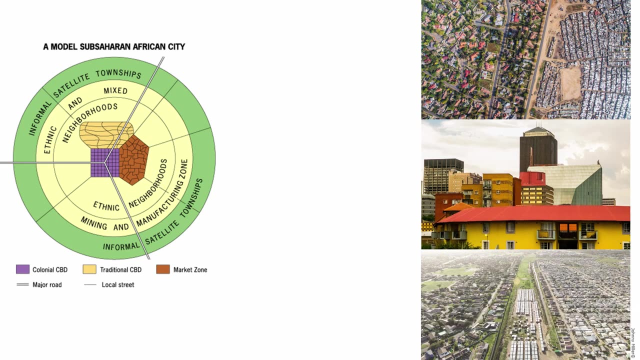 due to the fact that this region is heavily dominated with islands and peninsulas. The last foreign model is the Sub-Saharan African city And for this model, it's important to recognize that ethnicity plays a huge part, due to the colonialism that African countries faced. 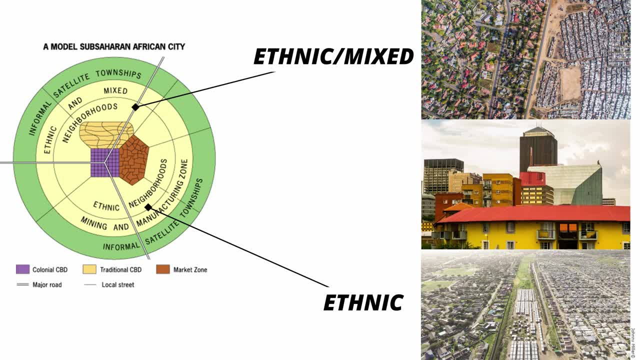 in the 19th and 20th century And in some parts you still see remnants of apartheid. It's not very uncommon to see ethnic and mixed neighborhoods being generally wealthier and the ethnic neighborhoods consisting of the shanty towns or squatter areas. 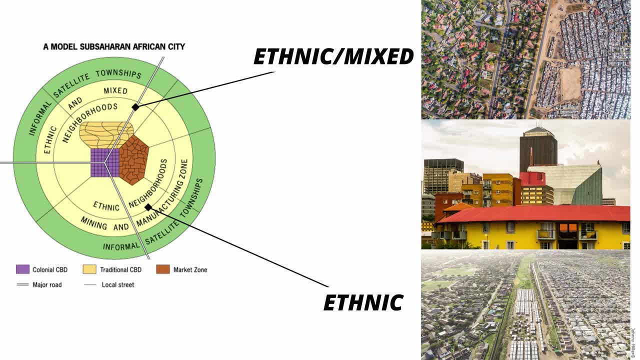 As you can see in the picture, these two areas tend to be divided, with your major roads or local streets, And in this model you'll also see three decentralized CBDs. Your colonial will consist of skyscrapers. your traditional with your lower density commercial. 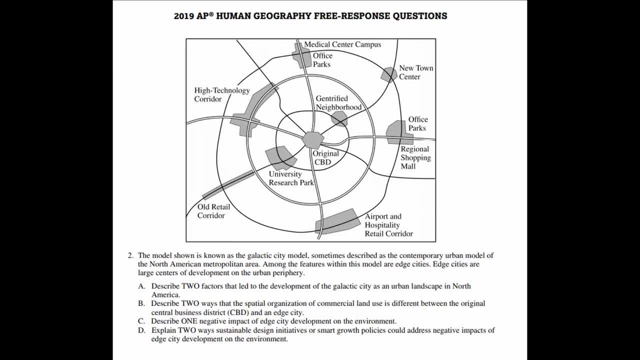 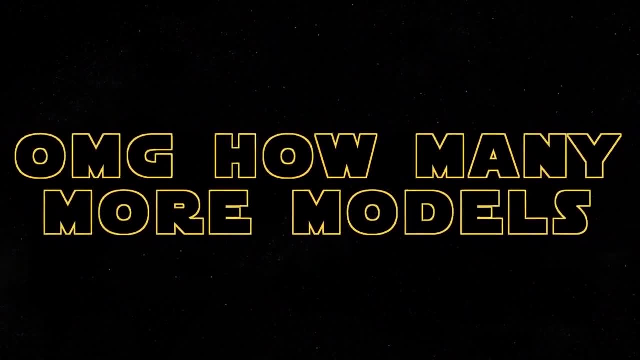 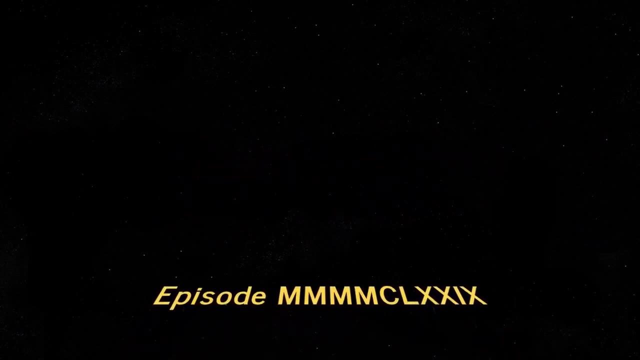 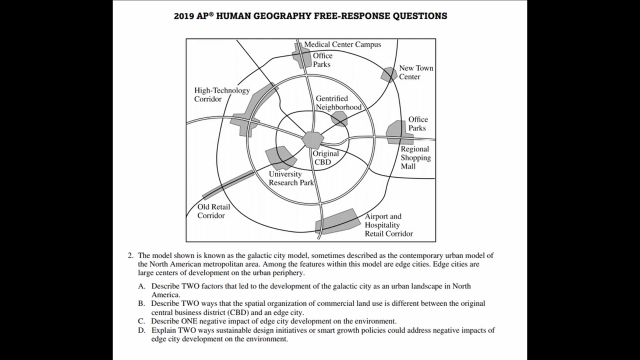 and your market zone with your informal markets. Lastly, the galactic city model. This model includes a combination of edge cities with various regions of specialization, which demonstrates decentralization, and they're loosely connected by freeways. And by the end of this section, you should be able to answer this practice FRQ. 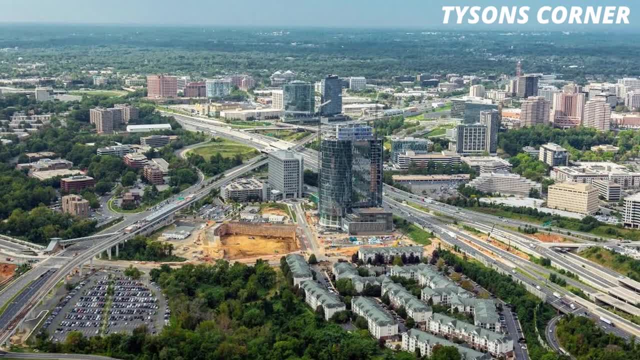 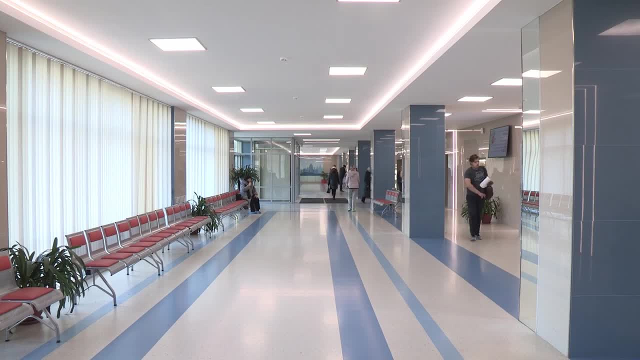 so feel free to come back to it. A really good example of an edge city is Tyson's Corner, and edge cities are large nodes of retail activities such as malls, medical buildings and commercial offices on the edges of an urban area Due to its commercial nature sometimes, 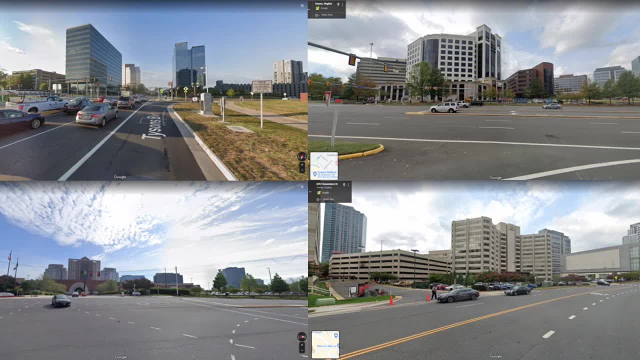 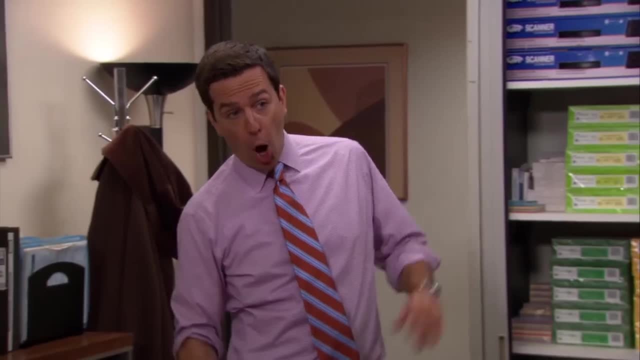 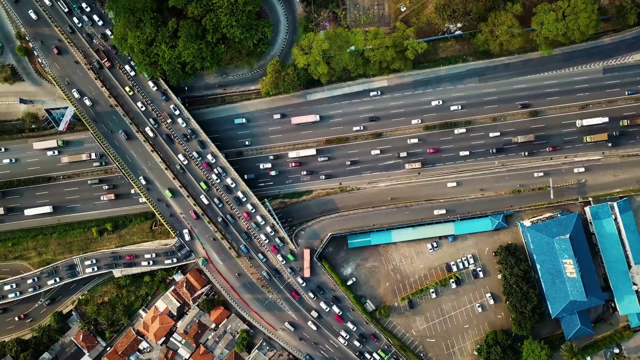 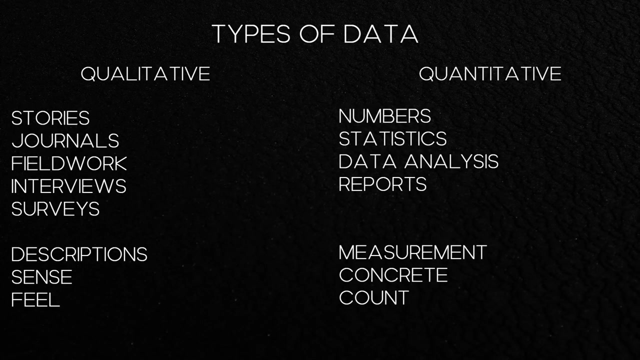 after businesses close, edge cities can lose population at night as people drive back to their homes in other regions. Because edge cities are connected by freeways, this can lead to increased traffic, which is directly correlated with higher levels of carbon monoxide and pollution. Speaking of pollution, let's utilize this to learn about. 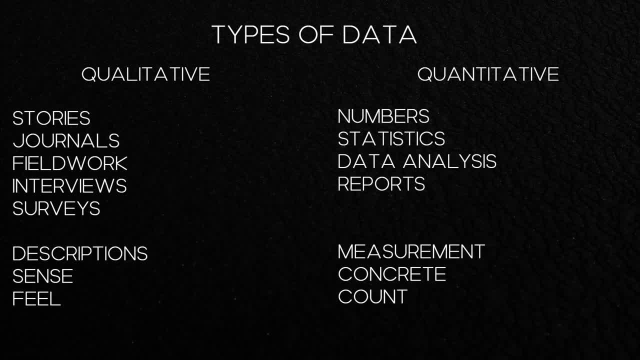 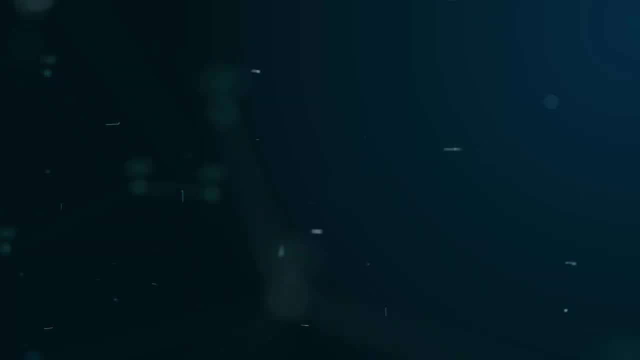 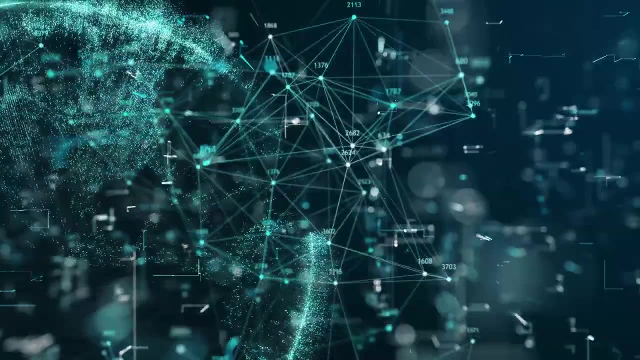 qualitative and quantitative data. Qualitative data includes interviews and first-hand accounts, whereas quantitative data includes statistics and concrete numbers. If you wanted to obtain quantitative data on traffic, for example, you'd look at the number of accidents in a city, count the number of traffic tickets. 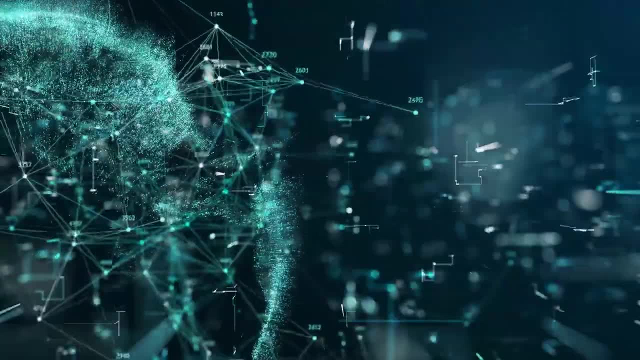 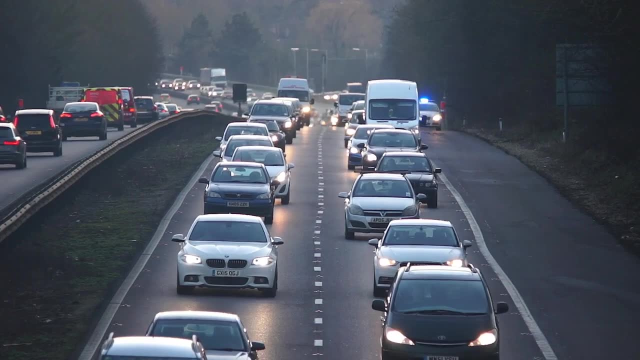 or even measure CO2 emissions in the atmosphere. Qualitative data, on the other hand, would consist of interviews on how long it takes people to get to work or fieldwork in downtown areas to look at average traffic speeds. And now let's move on to zoning In zoning. 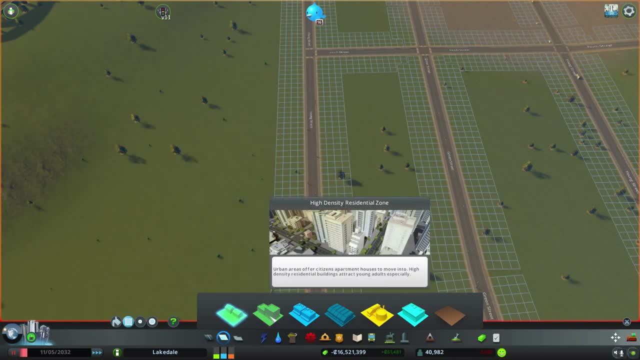 there's low-density residential, so your houses. Then there's the high-density residential, your apartment complexes or sometimes even your condos. You have low-density commercials- so think of your 7-Elevens or single-story offices- And finally you have your high-density. 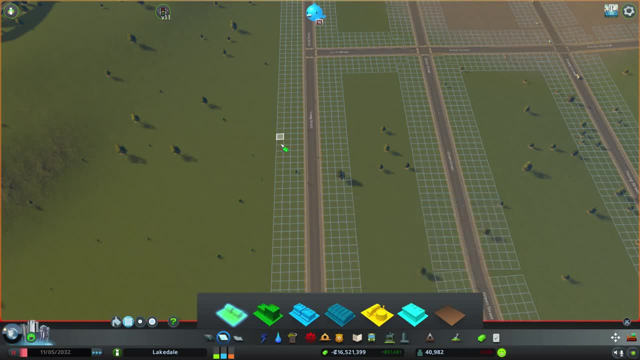 commercial, and that includes skyscrapers with offices. Although you can't see it, your city actually dedicates certain regions to certain zones, and quite a bit of urban planning is done around your city. Speaking of zoning, I would be remiss if I didn't talk about 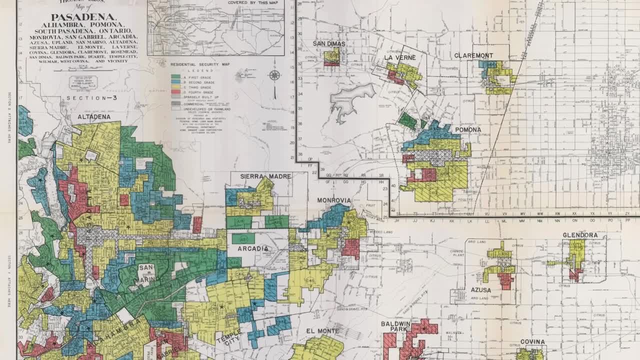 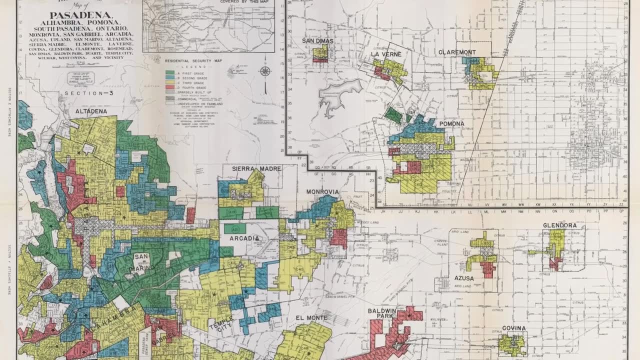 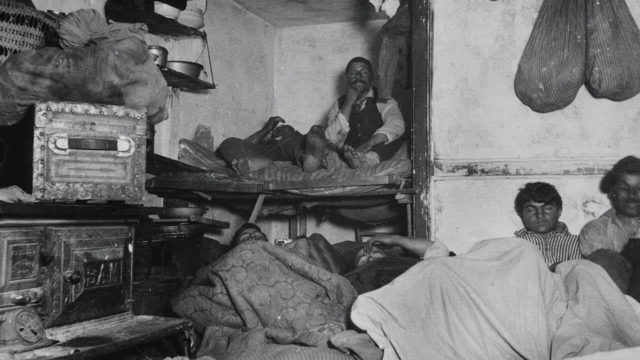 redlining, a practice in US history that restricted certain zones for minority groups in order to limit housing opportunities in wealthier neighborhoods. In order to understand redlining, you must understand the history of US suburbanization, which began with the large influx of immigrants near downtown areas As city centers became overpopulated. wealthier Americans. 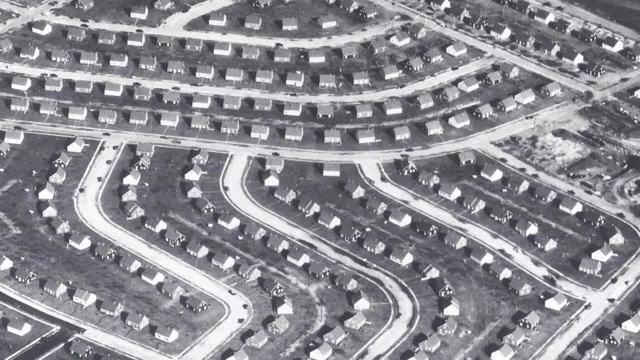 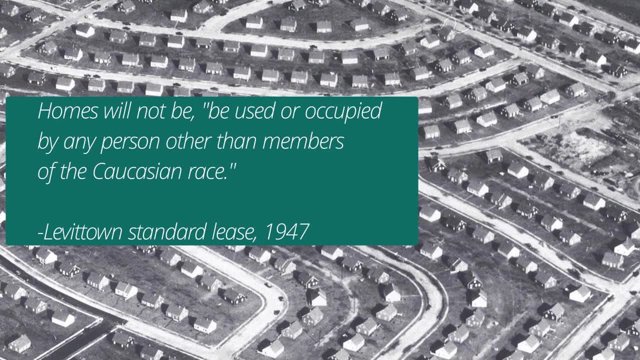 who tended to be white, moved out of the city and moved into the suburbs, with the first being Levittown, And here's a quote from the Levittown Standard Lease. it essentially stated that minority groups couldn't buy homes there. However, 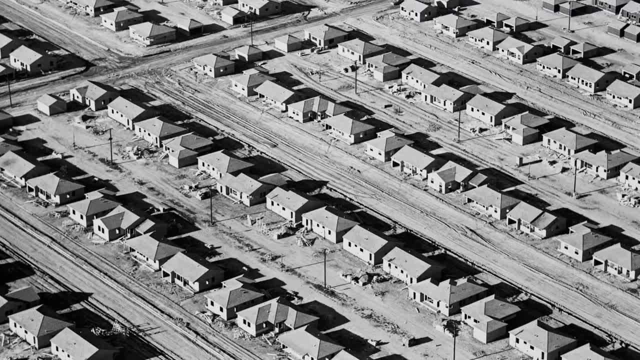 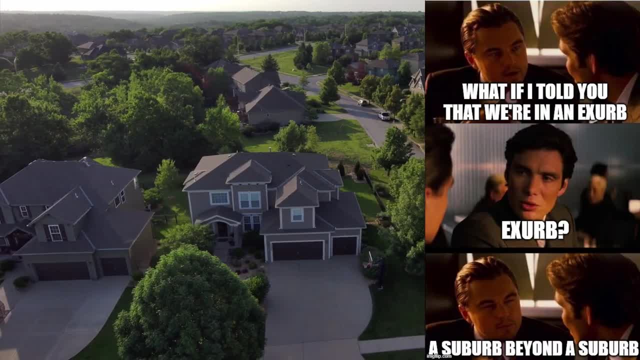 suburbanization continued on and eventually, in 1968, redlining was outlawed. The suburbs would take on various forms and they would include the exurbs, which is a suburb beyond the suburb, and a boomburb, which is a suburban region that has exploded in growth. 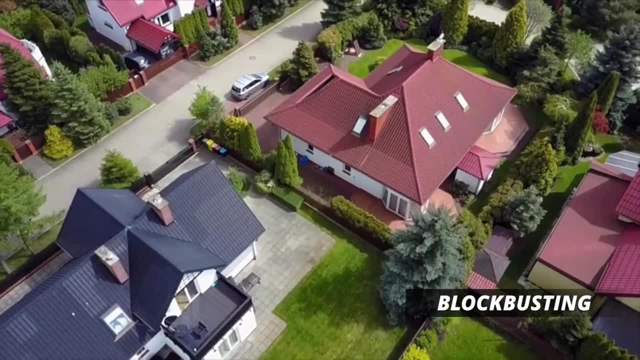 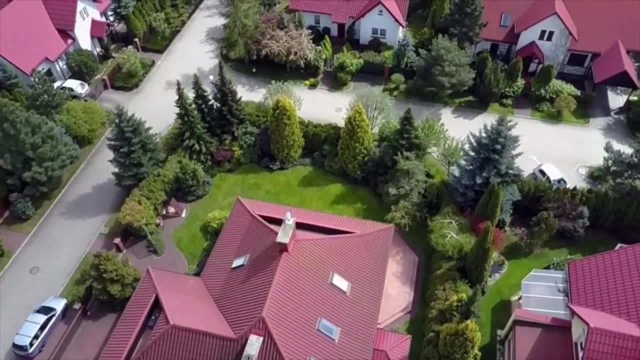 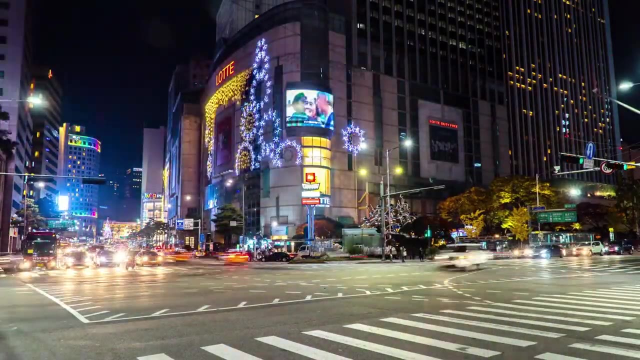 Another discriminatory practice that was utilized was called blockbusting, where real estate agents would convince white homeowners to sell their houses for cheaper by telling them that minority groups were moving into the area. When there's massive amounts of growth for urban or suburban areas, the primary concern becomes urban sustainability. Concerns surface about whether 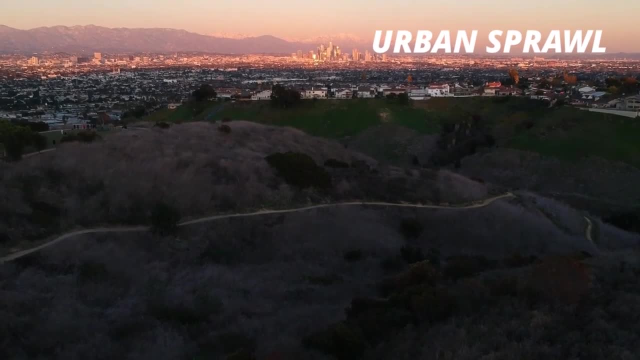 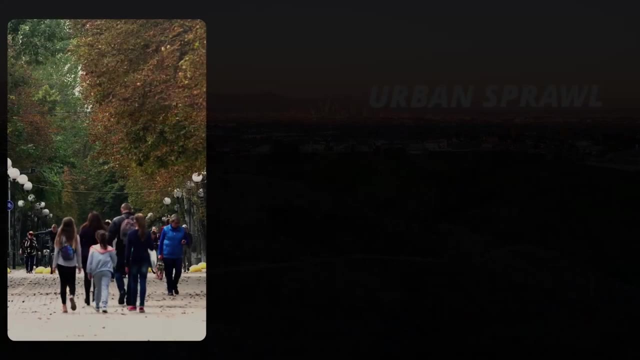 or not this amount of urban sprawl and the pollution that comes along with it is sustainable. Geographers and urban planners have responded by promoting urban walkability, a push for public transit like buses and trains, and a specific strategy they've utilized is called. 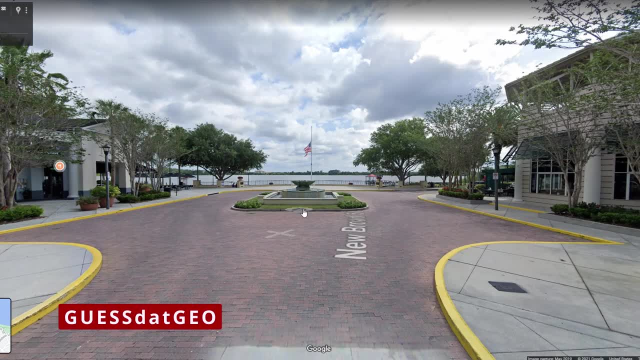 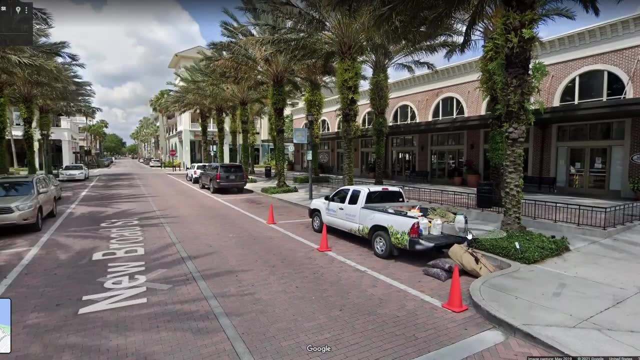 new urbanism. In today's episode of Guess That Geo, not GeoGuessr- I don't want to run into a lawsuit- We got this area, which is next to a lake. We have some palm trees next to sidewalks and on the left hand side, right here, we have a pretty 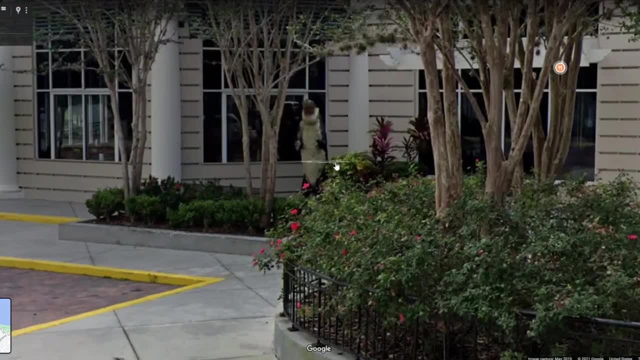 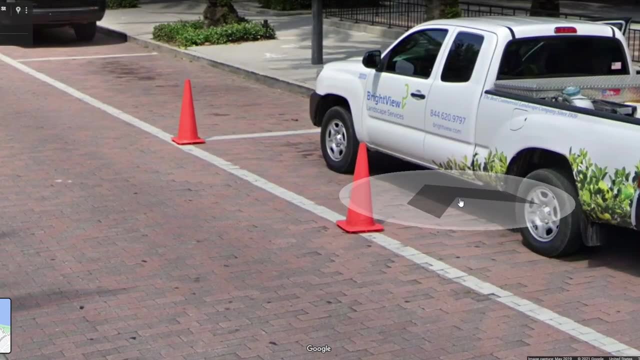 big clue: There is an alligator. So pause the video, make an educated guess and write that down in the comments below. According to my boy, GeoWizard, the key to this game- you gotta look at signs. That one's not very useful, but this one over. 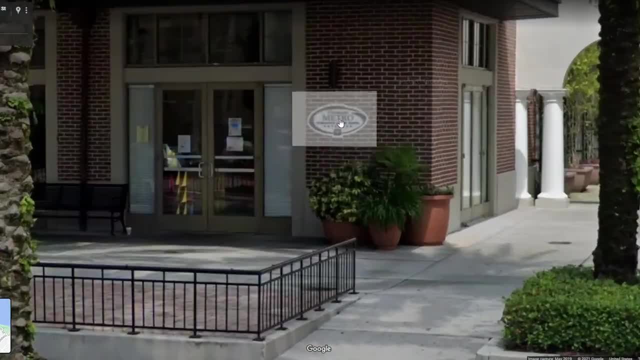 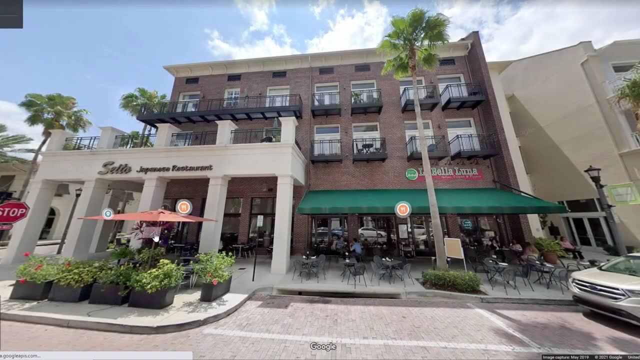 here says Orlando. So if you said Florida, congratulations, you can deem a Lamborghini of your choice. So this is Baldwin Park in Florida and we see examples of new urbanism here, with the commercial down below and the residential up top. 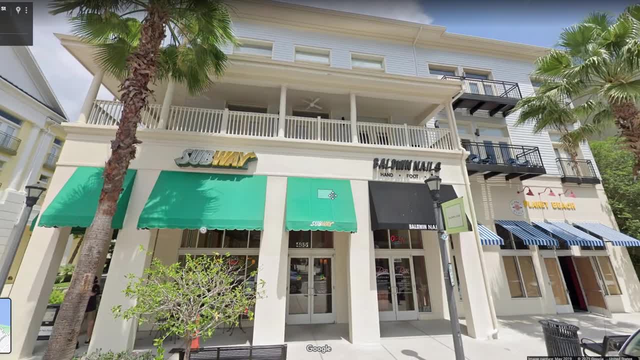 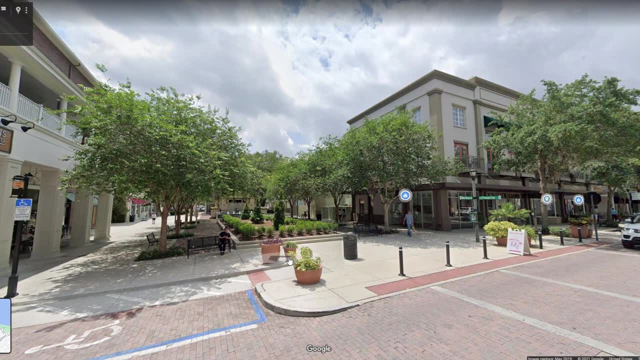 Here's another example, with the subway down below and the residential up top, and if we just turn around, we're gonna see that this place emphasizes walking areas, small plazas, emphasizes trees and grass and limits car use by making streets smaller and much more narrow. 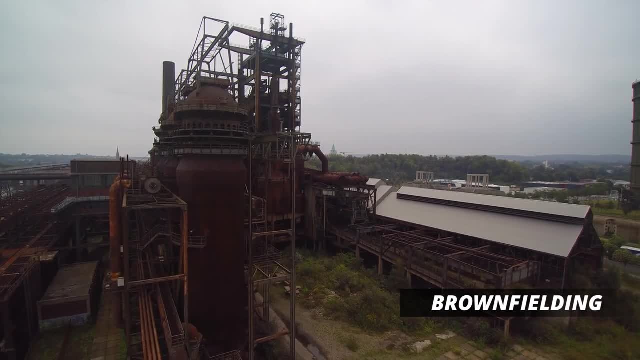 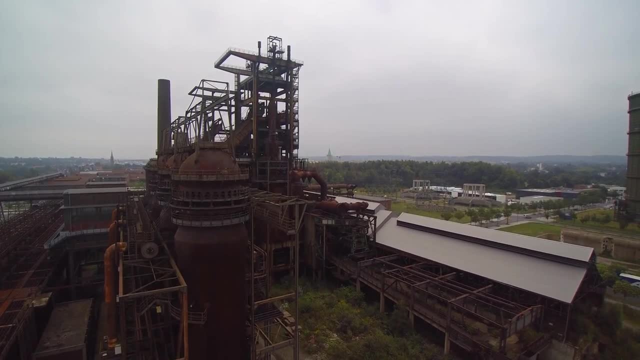 Another method utilized to prevent sprawl is called brownfielding, the process of redeveloping rusted factories into usable urban areas. You can redevelop this area into a mall. you could create a shopping center or even an apartment complex. Geographers also utilize what's called a greenbelt. 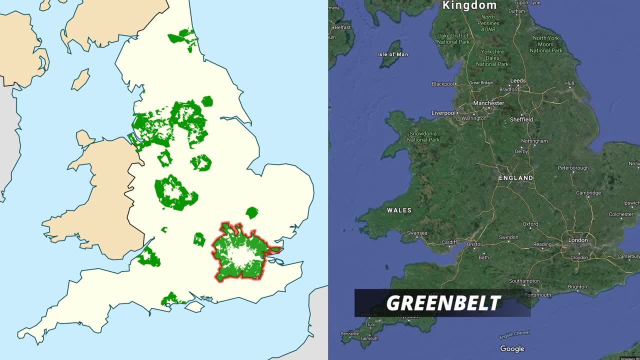 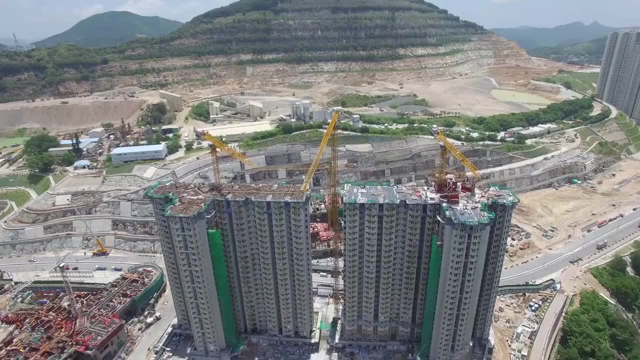 which is the process of surrounding a city with trees, forests or even with farmland, and Canada uses this strategy quite often, and London is a really good example of a greenbelt. And then there's infilling, and this could come in the form of filling in empty spaces or increasing. 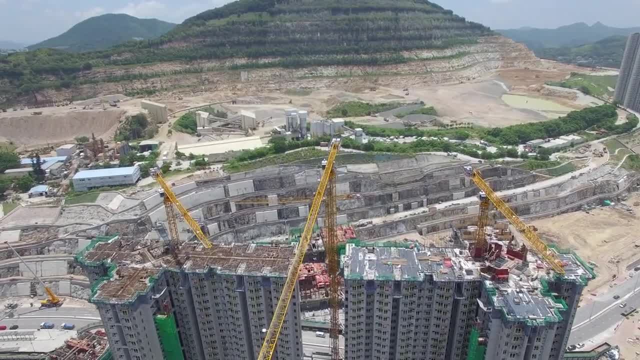 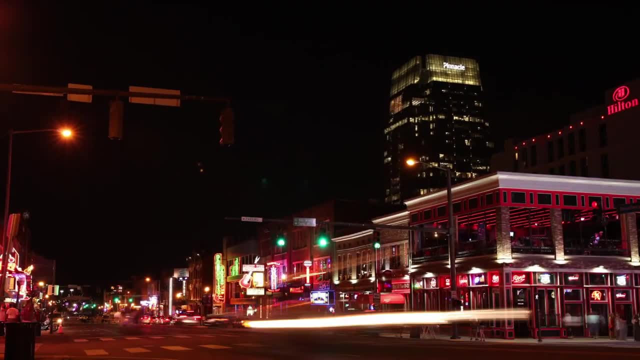 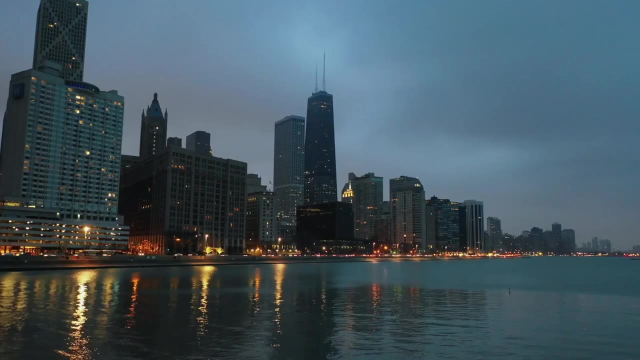 density within a region. For example, if a property owner was to destroy a single family home and create an apartment complex, that would be infilling. Although all the mentioned methods sound like amazing plans to create urban sustainability, they do come with their share of challenges. When you implement new urbanism or redevelop an area, that area can 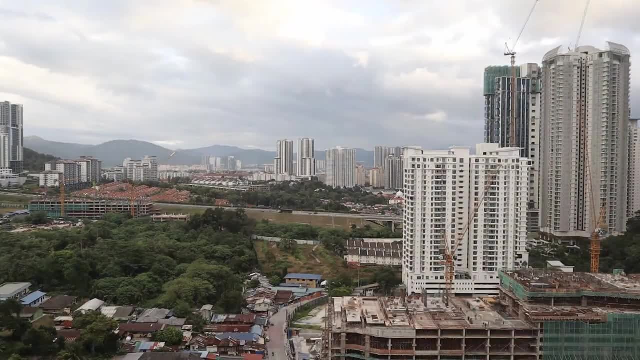 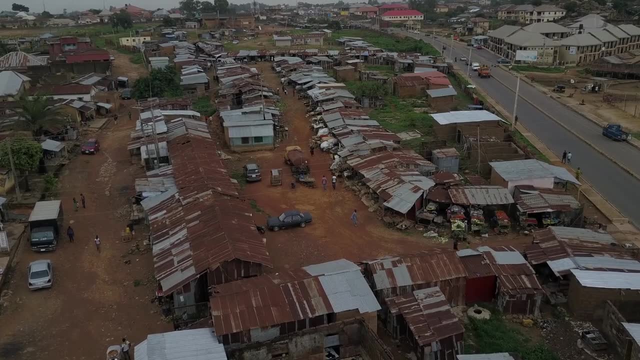 experience gentrification, which is the process of increasing land costs and property values. That sounds great, but this can lead to de facto segregation or indirect segregation, as lower-income residents who lived in the poorer areas prior to the redevelopment can no longer afford to live. 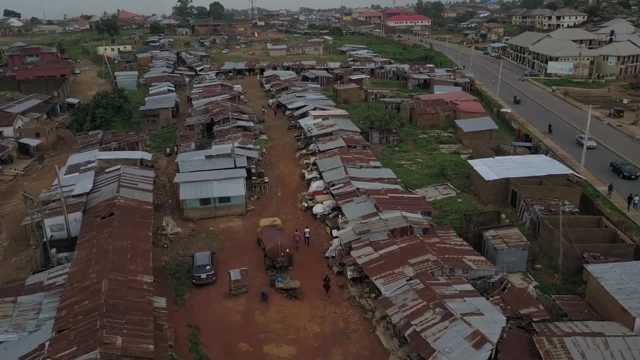 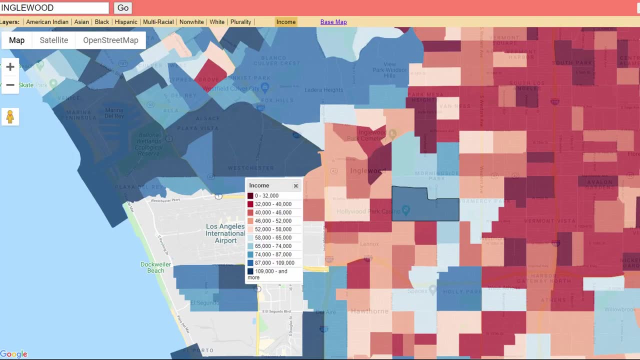 there as rent becomes more expensive and you also risk potentially losing historical place for characters. This is happening with the creation of the LA Rams SoFi Stadium in the city of Inglewood. Here is an income map of Inglewood and the blue represents higher. 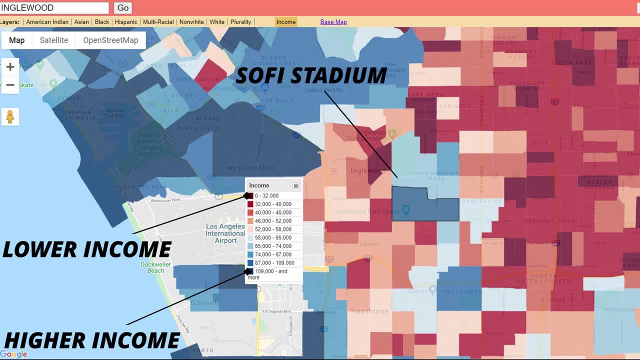 income and the red represents lower income. and this is the exact location of this stadium. Notice how it is a blue region that is now surrounded by lower-income areas. eventually, these areas around here can experience gentrification and lose their cultural identity. 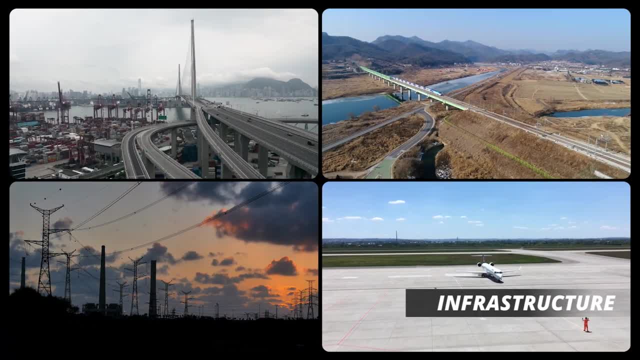 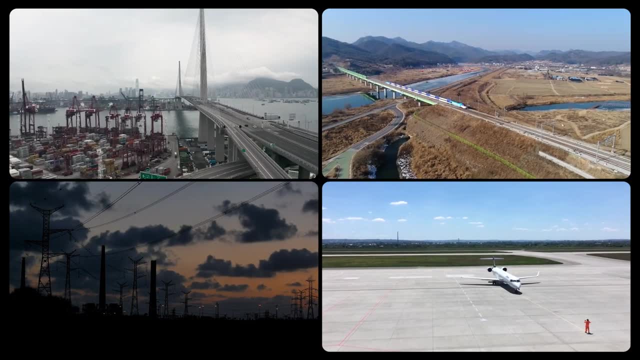 And finally, in reference to development, we have Economic infrastructure, which includes bridges, roads, public transit, power lines, airports, and you need to understand that all of these contribute to economic development of a city because they establish the foundations for jobs. 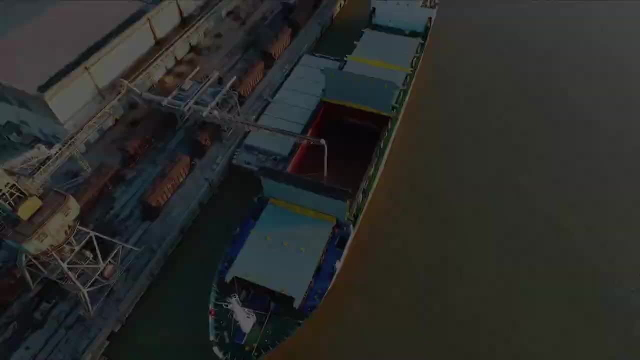 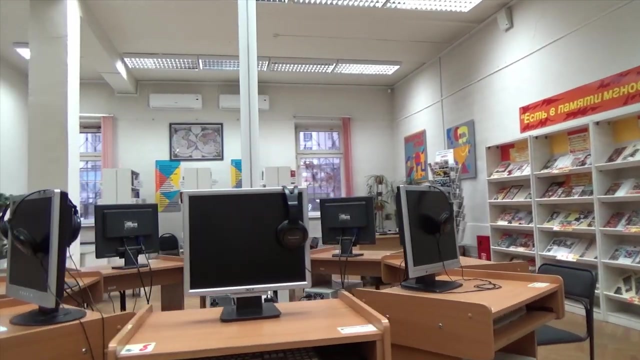 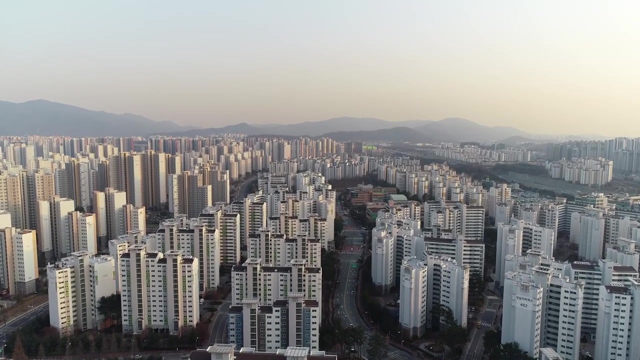 trade and development. and then you have social infrastructure, which includes schools and hospitals, and they contribute to the social development of a region by educating your population and establishing a sense of community. Alright, that is it for urbanization. I appreciate you all for tuning in. If you haven't seen the